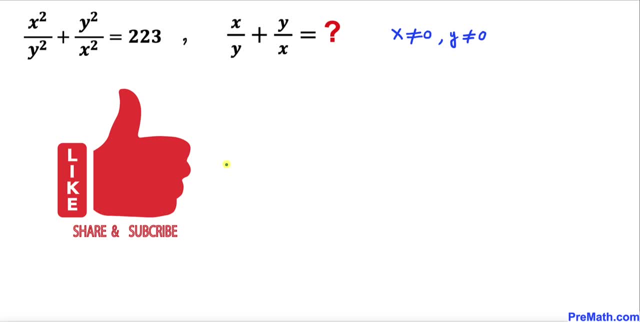 as well. Please don't forget to give a thumbs up and subscribe. So let's go ahead and get started with the solution, and here's our very first step. Let's recall our this famous identity: a plus b, whole square. If we suppose that our a equals to x divided by y and b equals to y divided by x, 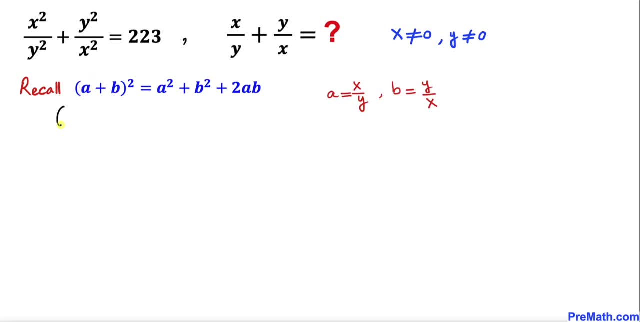 then we can write the solution. So let's go ahead and get started with the solution. write this equation as x divided by y plus y divided by x whole square equals to x divided by y whole square plus y divided by x whole square plus two times x divided by y times. 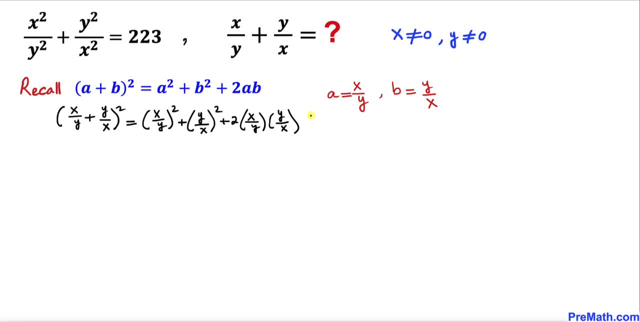 y over x. and now let's go ahead and simplify the right hand side of this equation. So x divided by y whole square could be written as x squared divided by y squared plus. likewise this could be written as y squared divided by x squared. and here x and x crosses each other out. y and y is gone, So we 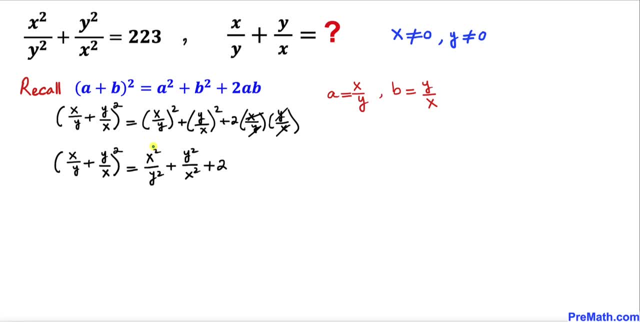 can write this equation as: x squared divided by y squared plus y squared divided by x squared is equal to 223 from this, our given equation. So therefore, on the right hand side, I'm going to replace this one by 223 plus 2, which is equal to 225, and now let's go ahead and get started with the solution. So let's. 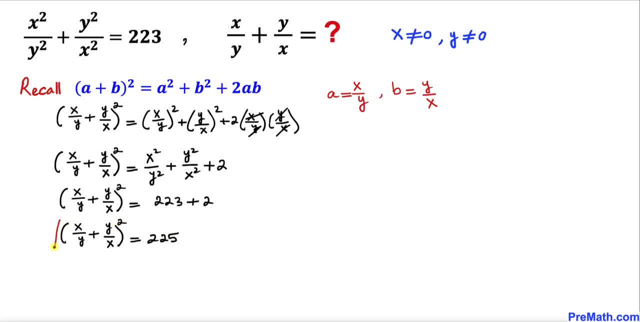 go ahead and undo this square by taking a square root on both sides of this equation. and here we can see that this square and square root, they undo each other. so we simply ended up with x divided by y plus y divided by x. turns out to be simply the square root of 225. is positive or negative, or?